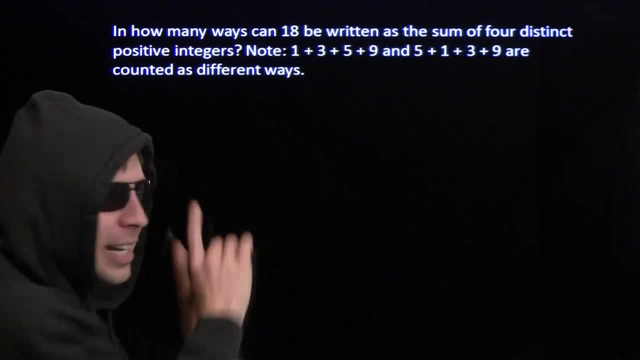 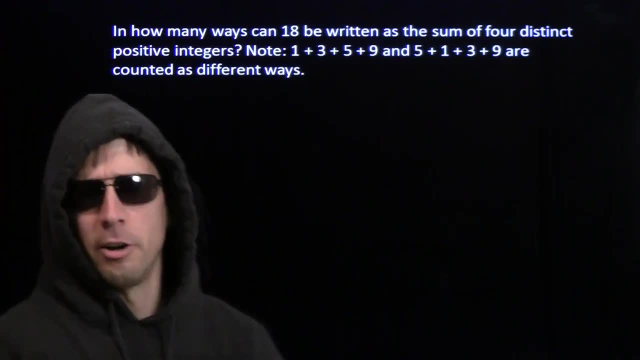 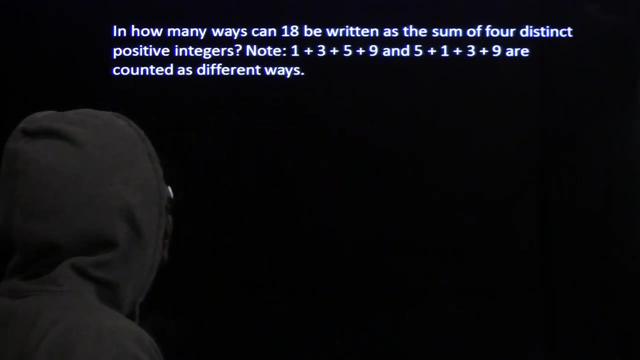 It's going to be cooler, Because that's what kind of guy I am. Now I'm going to start off by knocking this problem off, just the same way that other guy would do it. He'd start off like this. That's my staring in confusion face. I'm not very good at it. I'm not as good as he is because, well, he's got a lot more experience with it, But he'd stare at confusion for a little bit. Stare, stare, Be kind of stuck. We could at least make one interesting observation here, and that is well once we get one group of four. distinct, that means distinct. 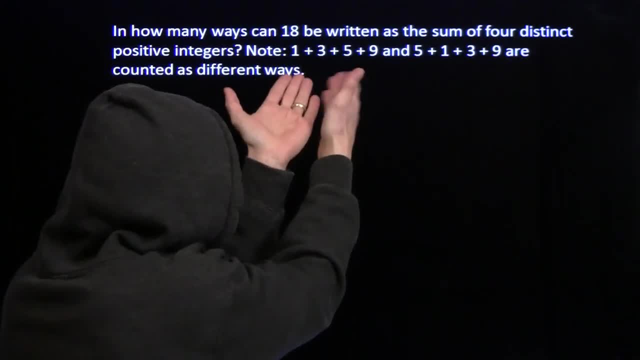 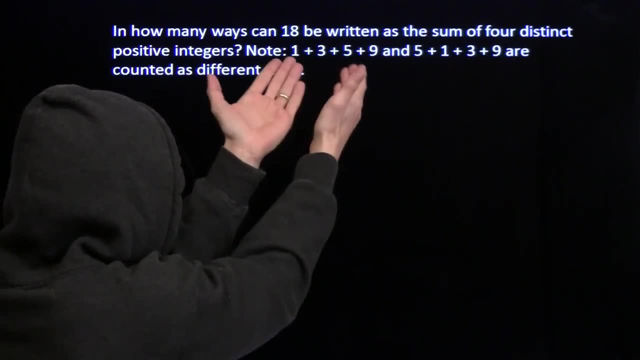 positive integers. well, we can get others by just rearranging these numbers. You know, rearrange this like this, you get another one. So once you get one group that works, we can just think about how many ways can I arrange these four numbers? Well, they're different. You, 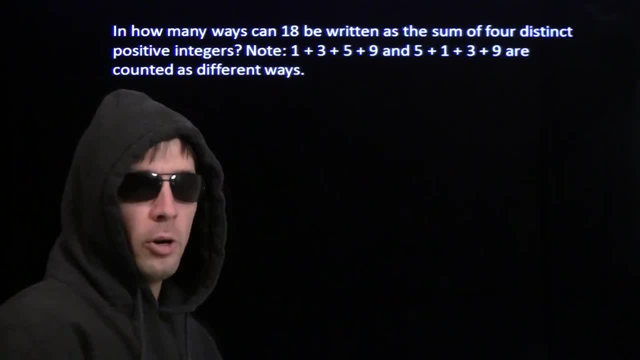 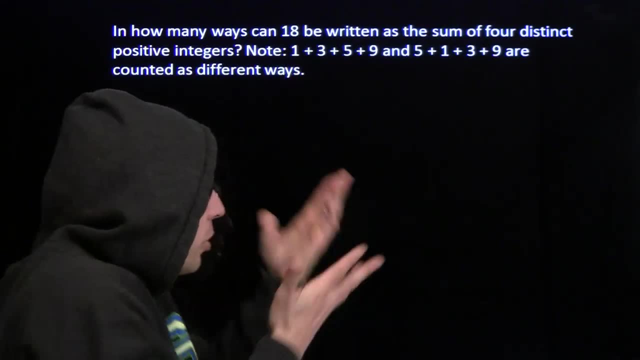 got four different things. How many different ways can you order them? in a row, That's just four, factorial, That's 24.. So now, once we find one group, we don't have to list out all those 24 orders. We know there are 24 of them. So now we've made the problem a little bit easier. We. 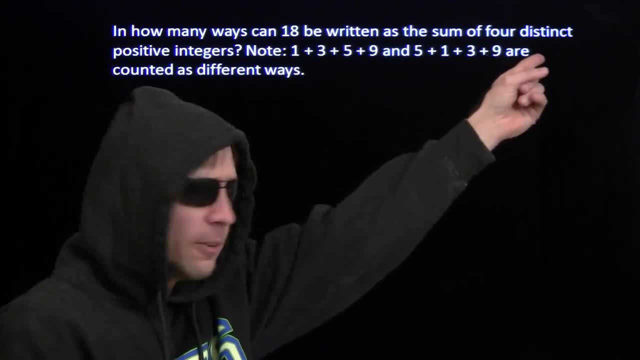 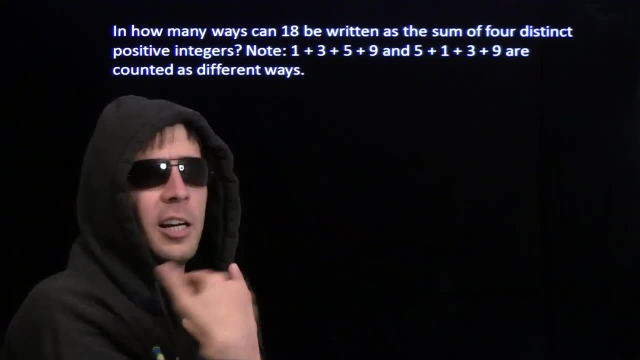 just have to find how many different groups of four numbers, four different numbers, add up to 18.. And once we've figured out how many of those groups there are, then we multiply by 24 to take care of all the different orders of the numbers in those groups. And now how to count the number. 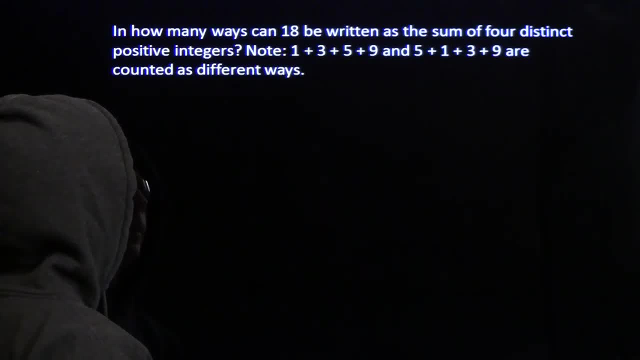 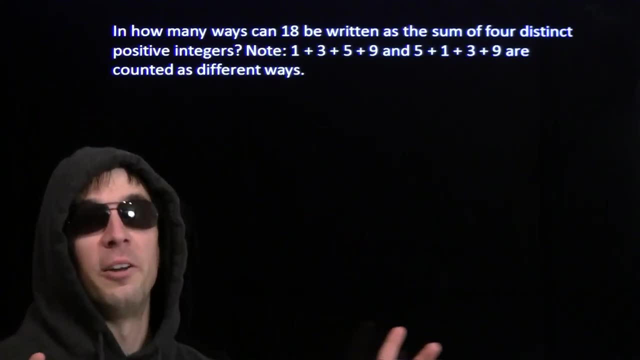 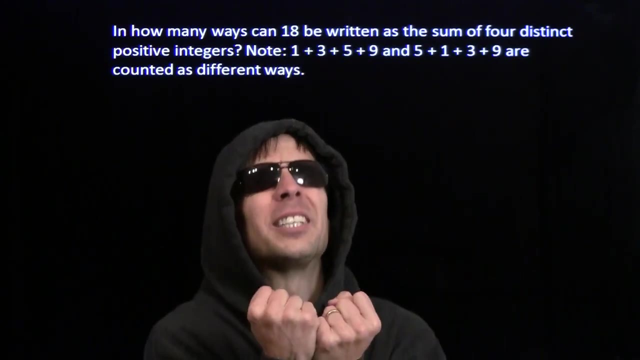 of groups there are- Now I'm stuck. That'll be the guy be like: oh, I'm stuck, Can't do anything smart. Then he'd break out one of my favorite lines: If you can't do something smart, then do something stupid. I love it when he breaks out that strategy because he's so good. 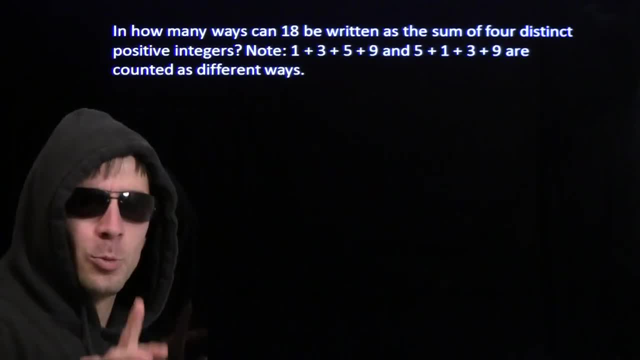 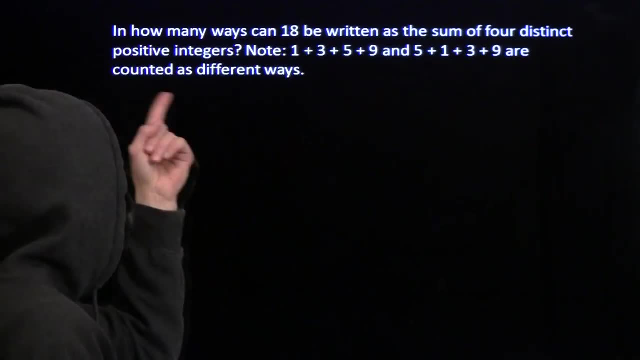 at doing stupid stuff. Oh, he's really good at it. And this is what he'd do. He'd say: OK, we're just going to list out the groups. We're just going to list out the groups of four distinct positive integers that add to 18.. Now, if you're going to do something stupid, you better be. 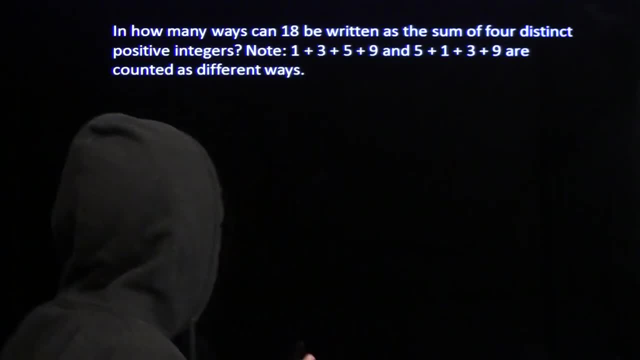 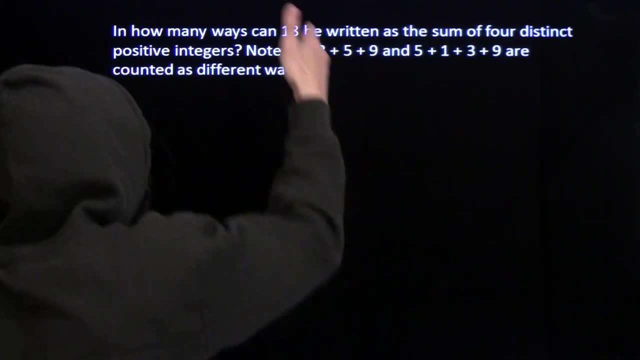 organized about it. If you're going to do something smart, you should be organized about it too, But it gets even more important when you're doing something stupid. We're going to be nice and organized in finding the different groups of four different numbers that add up to 18.. We'll start. 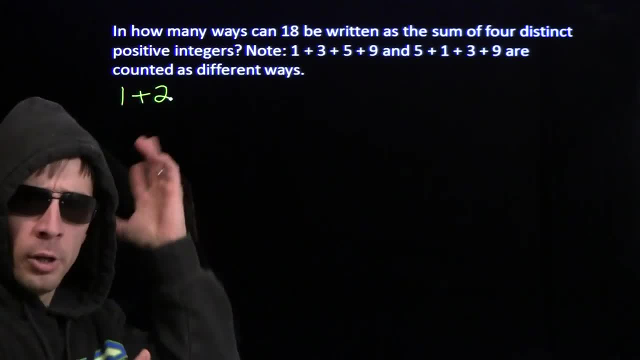 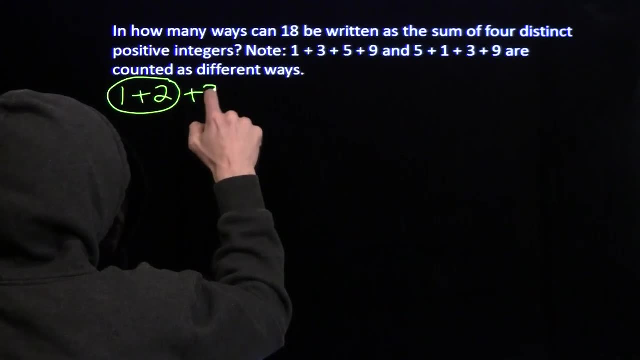 from the bottom. We'll start from 1 plus 2.. The groups that start off 1 plus 2.. And we'll go ahead and list out the ones we can find that start off 1 plus 2.. 1 plus 2 plus 3 is 6, plus 12 gets us up. 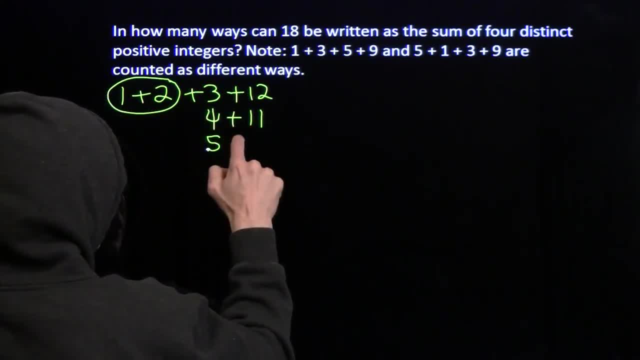 to 18.. And then we can just pound through these cases nice and quick: 5 plus 10,, 6 plus 9,, 7 plus 8.. And it's clear There are five that start off: 1 plus 2. And we box that off, We're staying. 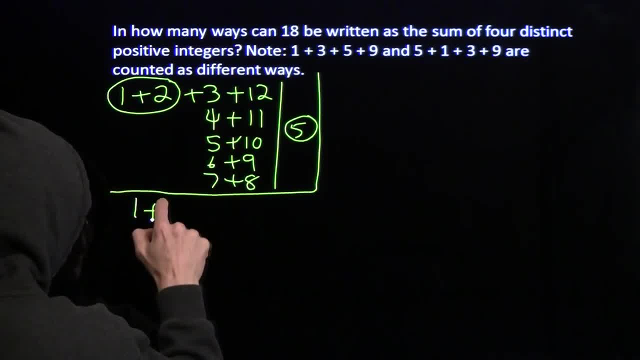 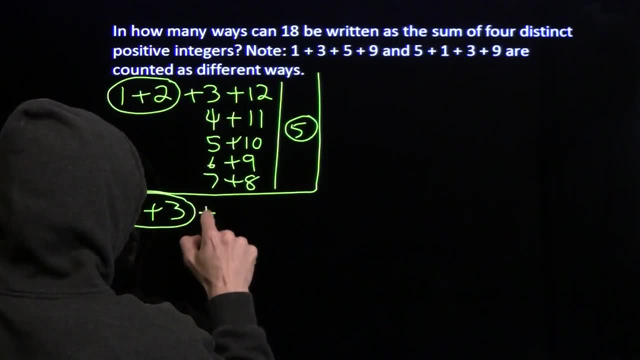 nice and organized And then we're going to move on. Nice, clear-cut, organized casework. And that's the key to getting through casework problems is be nice and organized, because then you can be sure that you've counted everything once and only once. You don't want to count. 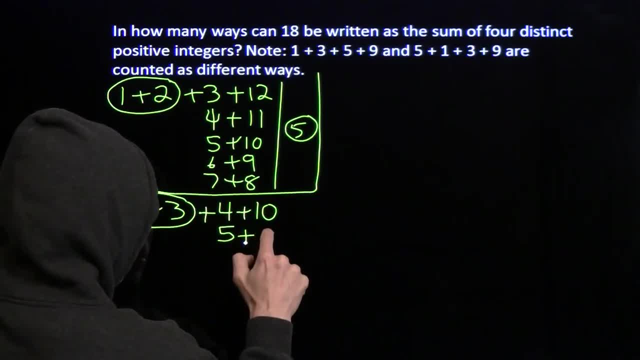 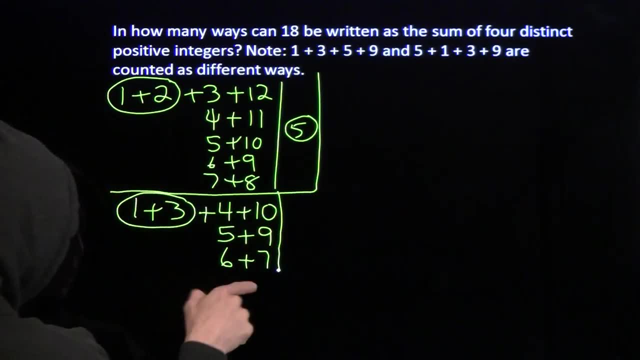 anything twice and you don't want to miss anything. So by being nice and organized, which is what we're doing, by starting from the bottom and working our way up, we can make sure we don't miss anything. 6 plus 7,, that's 6 plus 8.. 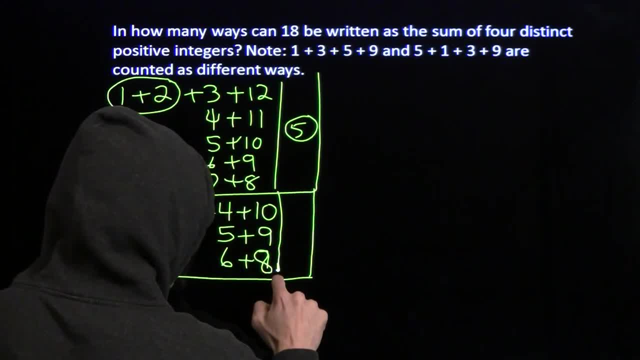 Bet the other guy wouldn't have caught that 1 plus 3 plus 6 plus 8 is 18.. We can't go up to 1 plus 3 plus 7, because then we'll have 1 plus 3 plus 7 plus 7.. Distinct means. 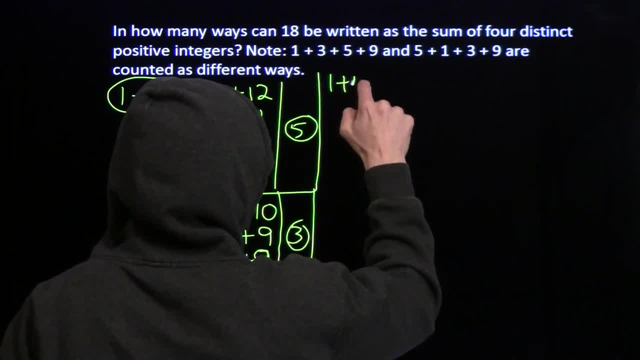 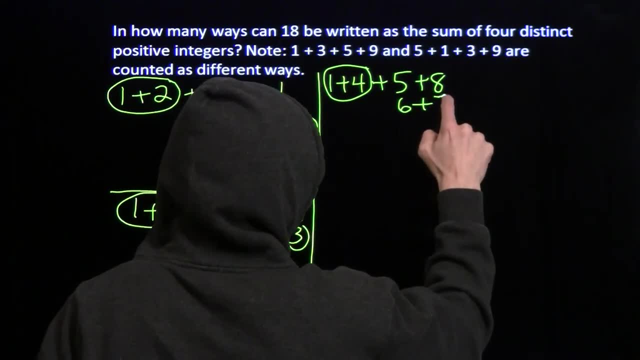 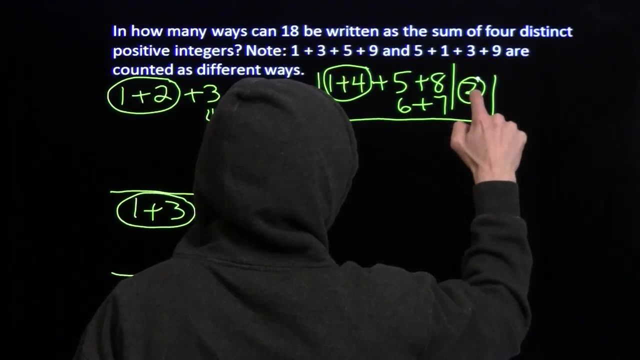 different. All right, Moving on to 1 plus 4. And then we go to 5. And then we add 8.. 1 plus 4 plus 6 plus 7.. No more Can't go anymore with 1 plus 4.. That gives us 2 more right there. Then we'll start. 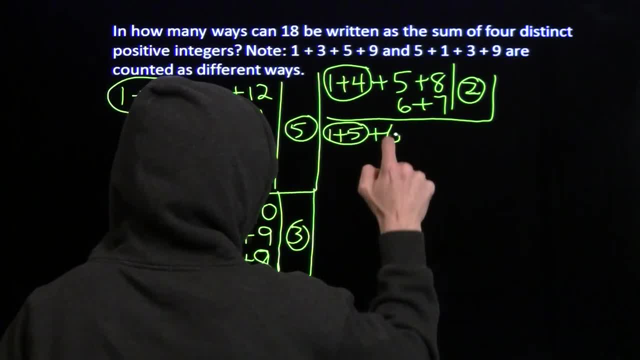 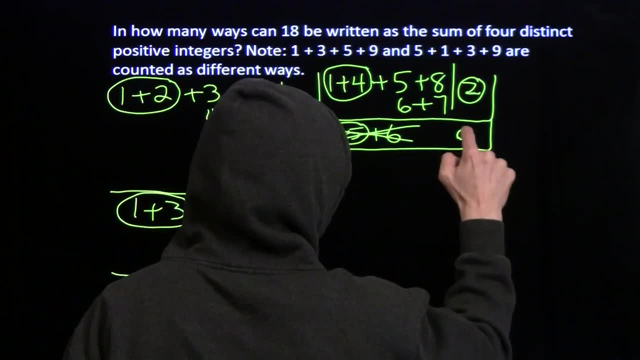 off with 1 plus 5.. 1 plus 5 plus 6. That gives us 12 plus 6.. Ah, you can't do that. Distinct means different. I know all about different. There are none in this case. 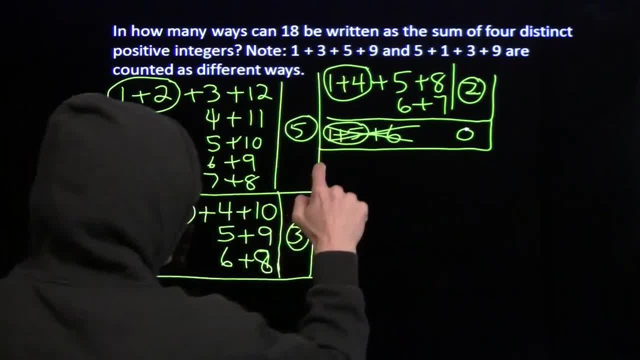 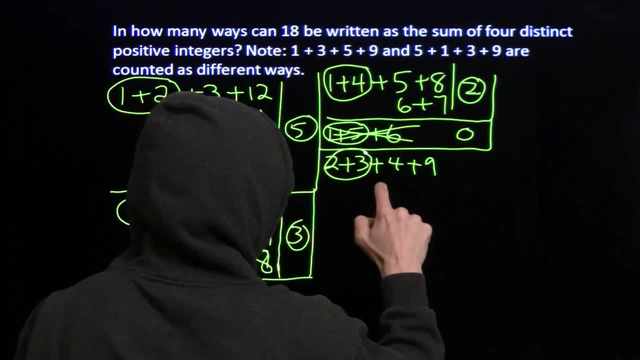 So we can't get anymore. starting with 1. We're going to move on to 2.. We're going to start off with 2 plus 3 plus 4 plus 9 plus 5.. 5 plus 8 plus 6 plus 7, we've got 3 more in this case. 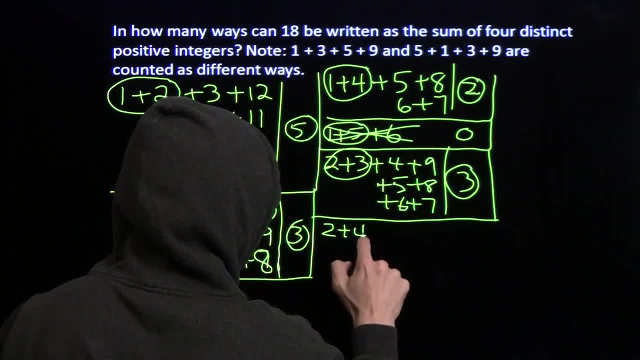 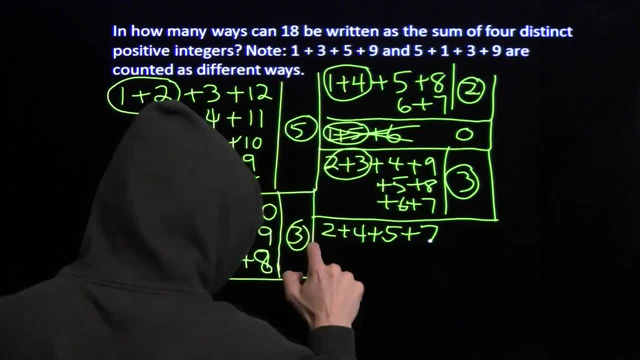 And we're moving on to 2 plus 4 plus 5, that gives us 11.. We need 7 more. We can't go up to 6 and 6.. Distinct means different. We've got 1 more in this case. 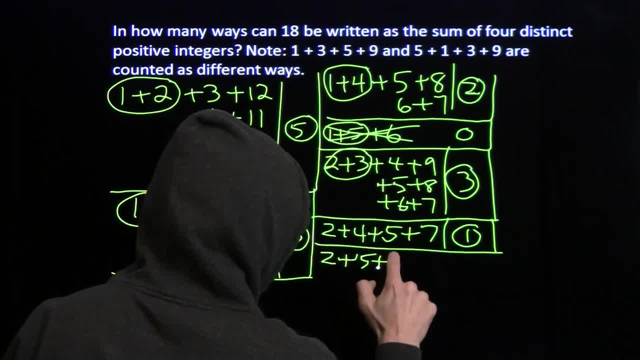 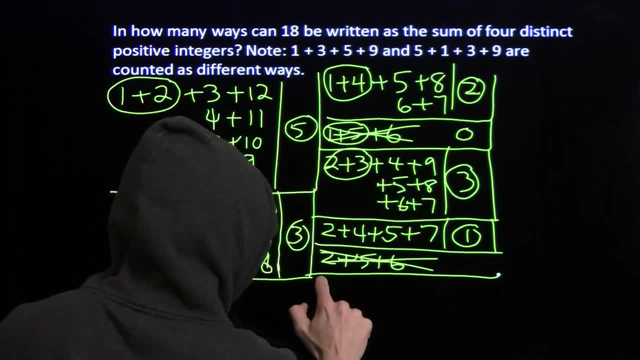 Now, if we start off, let's see we go 2 plus 5 plus 6, that gives us a 13,. we need another 5.. Ah, can't do that, Okay, And then now we can't do any more, starting with 2, so we're going to move on to 3 plus 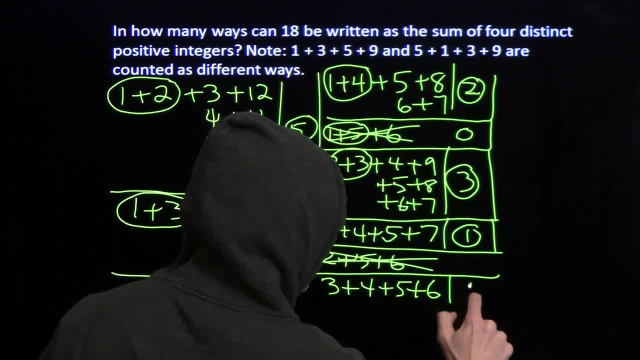 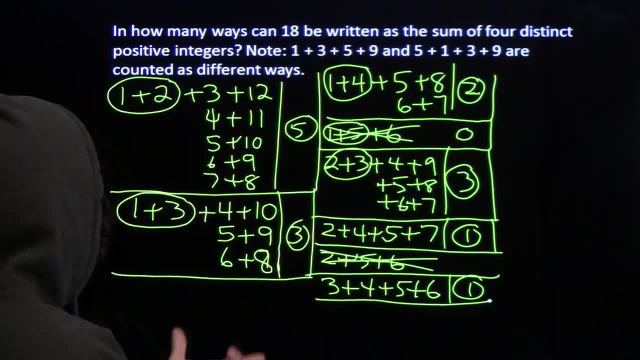 4 plus 5 plus 6, that adds up to 18.. That gives us another one, and clearly we can't get any more with 3, because we're going to get something that's larger than this, which means it'll be larger than 18.. 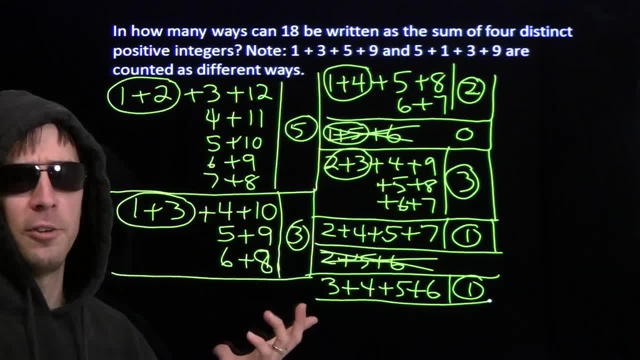 And if we tried starting off with 4, we go 4 plus 5 plus 6, we're already at 15. when we add on a 7, we're way past 18.. So look at our nice organized casework here. 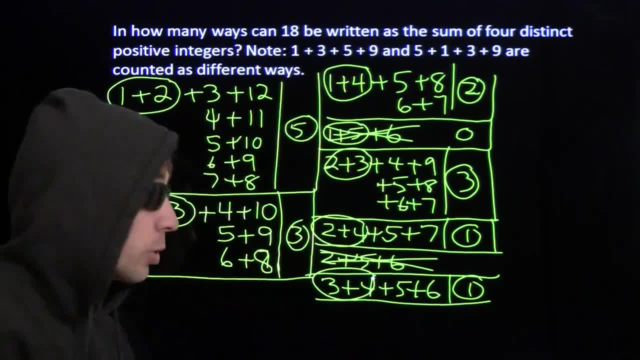 We took care of the ones things that start with 1, and the things that start with 2, and the things that start with 3.. We're just looking at the increasing groups of numbers, so we know that we've got everything. 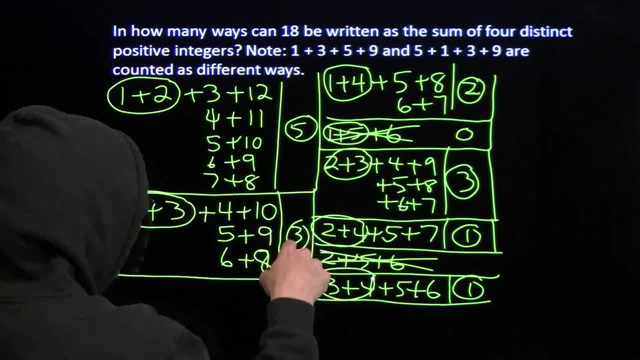 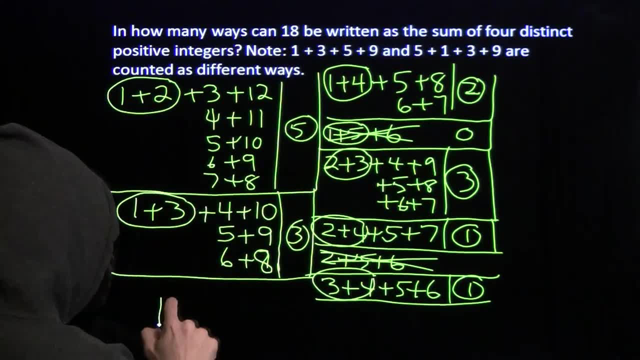 exactly once, and only once. We haven't double-counted anything. 5 plus 3 plus 2 plus 3 plus 1 plus 1, that's 15 different groups here, And then we have to multiply by 24, because each one of these groups, the numbers can. 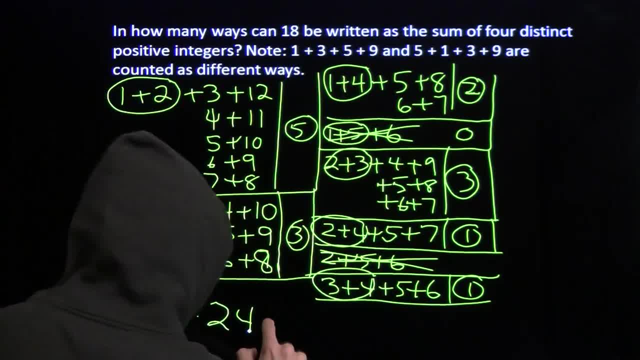 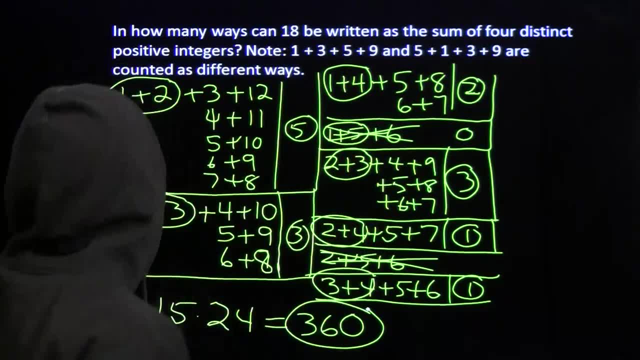 be ordered in 4 factorial. that's 24 ways. so we've got 15 times 24 is 360 ways. Okay, So we're going to take 4 distinct positive integers that add up to 18.. And see, this is where that other guy would stop. 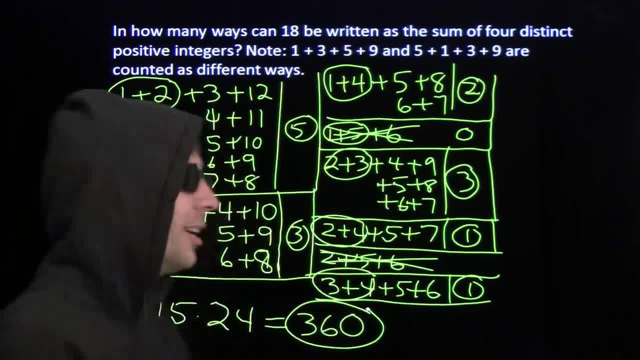 He'd be happy with this. He'd be like, hey, we did something stupid and we got the right answer. Not me, Not me. I said I'm going to change this problem just a little bit. Change this problem just a little bit. 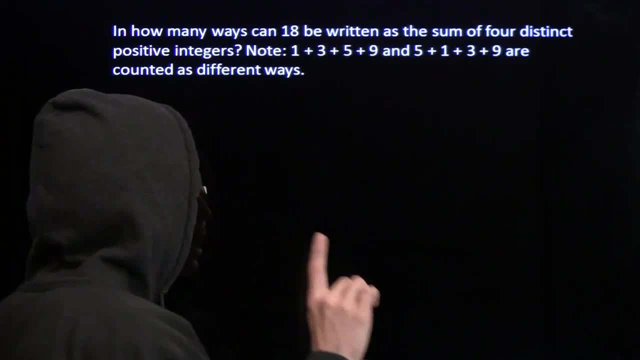 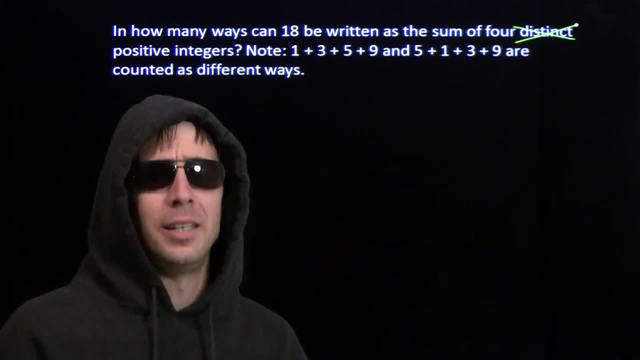 There's the problem again, and here's how we're going to change the problem. We're going to take out one word, just one word, and make it a completely different problem. We're going to take out distinct. It's different, but it's gone now. 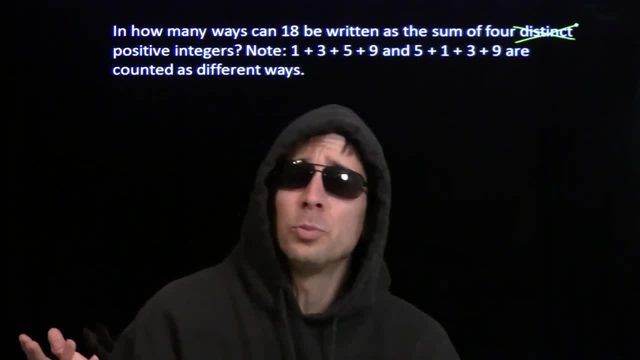 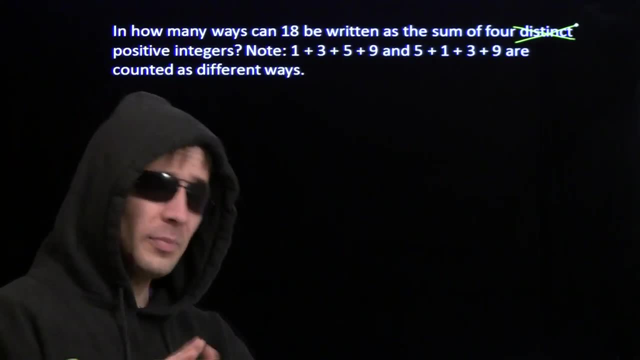 Now we just have 4 positive integers, add up to 18, so we can go 2 plus 2 plus 7 plus 7.. We can put that in this group, can't put it in the other one. So how are we going to tackle this problem? 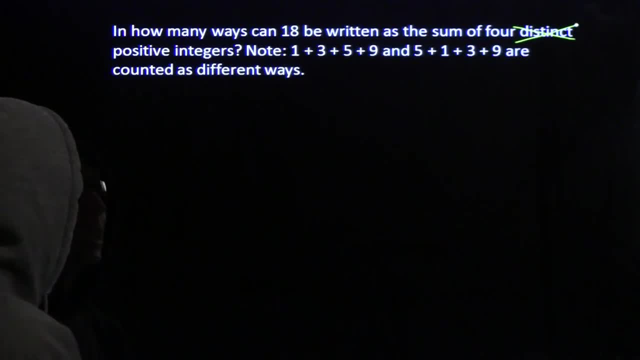 Now I'm going to start off just like that other guy would. I'm going to start off just like he would. I'm going to do something stupid. right, We're going to be nice and organized. We're going to do some casework. 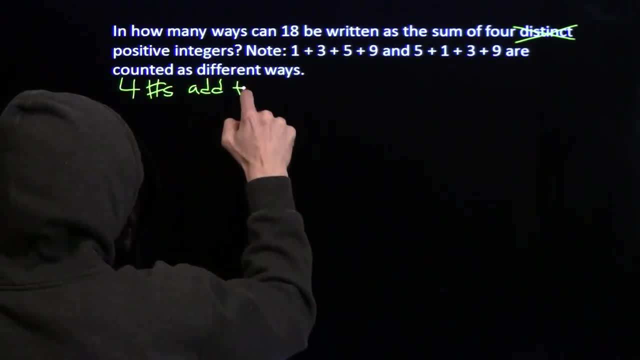 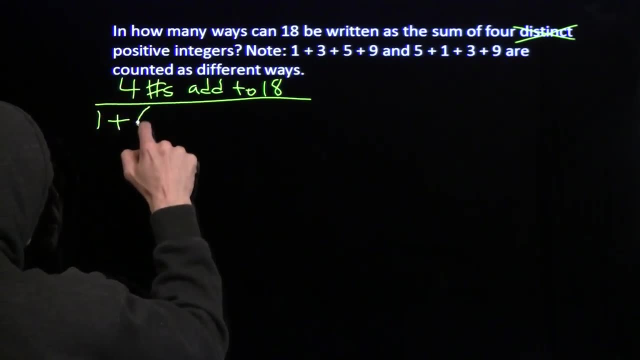 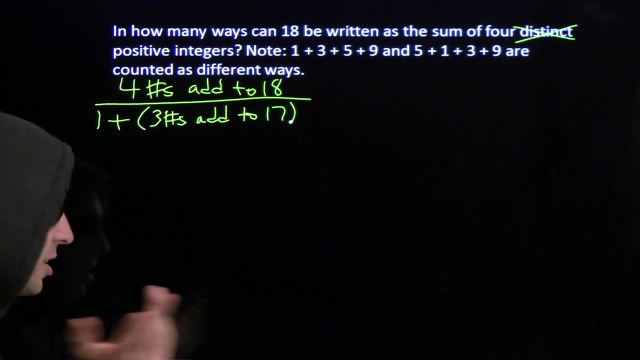 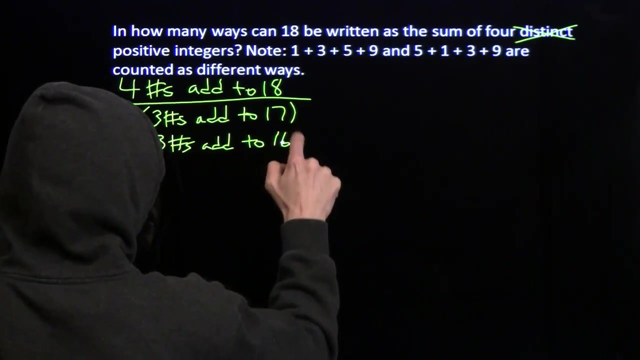 Four numbers that add to 18.. And once again, we'll start off low, work our way up. We'll go 1 plus 3 numbers that add to 17.. Next case, of course, is 2 plus 3 numbers that add to 16.. 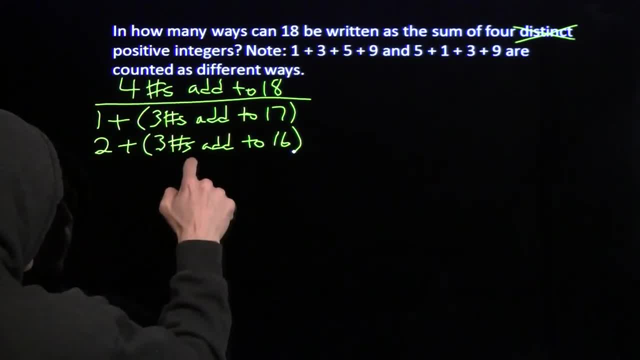 And then on and on down the line. 3 plus 3, numbers that add to 15, da-da-da-da-da-da. We keep on going, keep on going, keep on going, And eventually we're going to get down here. at the end we're going to have 15 plus 3. 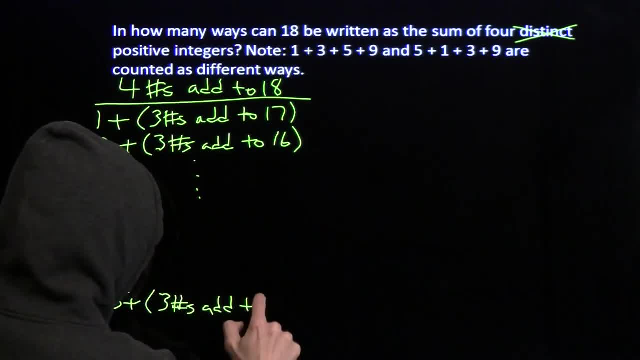 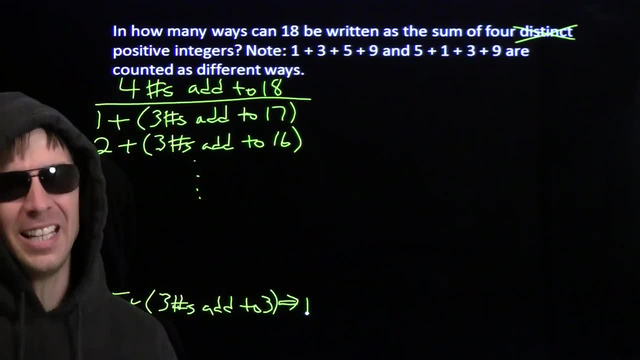 numbers that add to 3. That one's pretty easy. That's 1 plus 1 plus 1. Even the other guy would figure that one out. There's only 1 in this case, But we've got 15 cases. 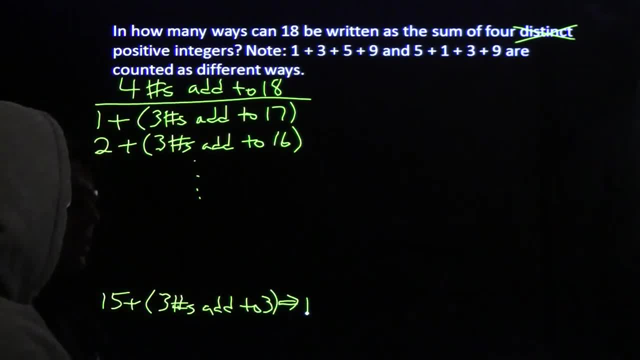 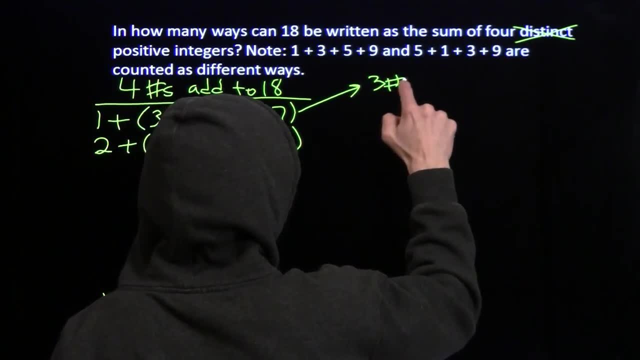 It's going to take a long time. Let's take a look at this first case right here just to get an idea of how long it will take. Take this first case: 3 numbers, add to 17.. All right, and be nice and organized. 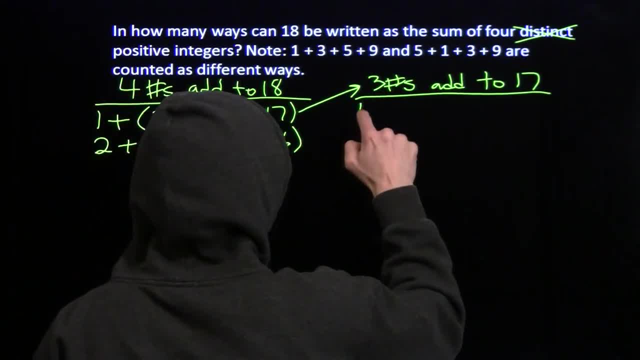 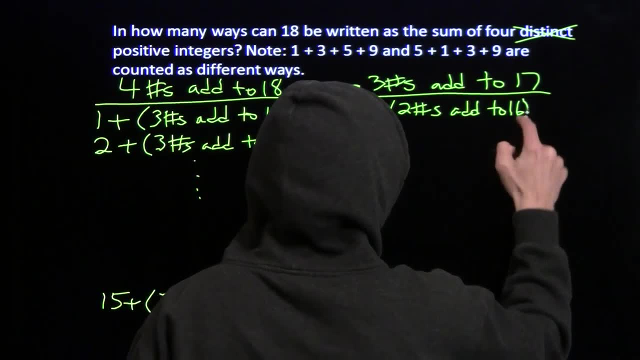 Again, we're going to break this one down into cases, And it's starting to look like we're going to be here all day. 1 plus 2 numbers, 3 numbers that add to 16. Well, at least that's pretty easy right. 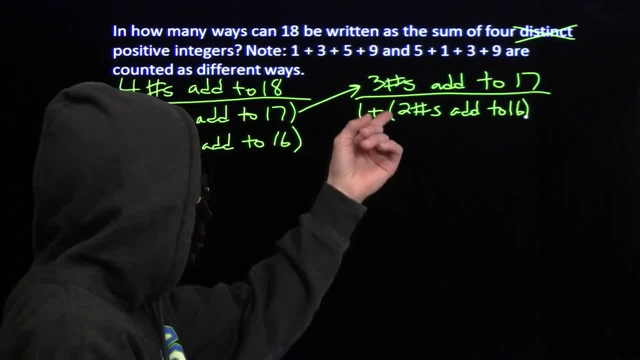 You can go 1 and 15,, 2 and 14,, 3 and 13, and so on. You know there are 15 different numbers you can pick. For your first number, you can pick anything from 1 to 15, then you automatically have. 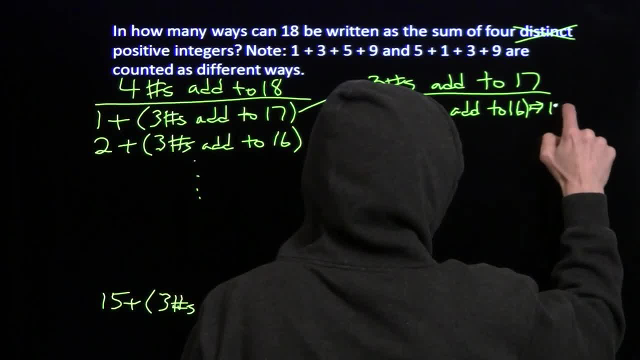 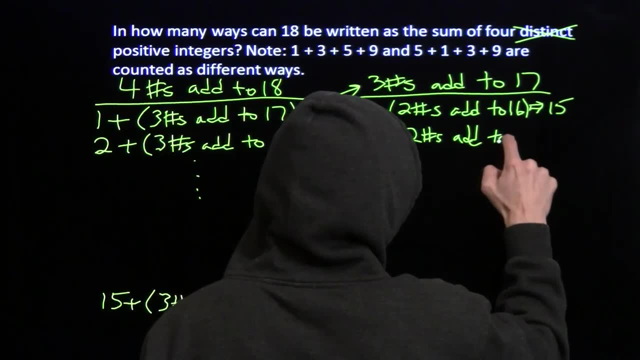 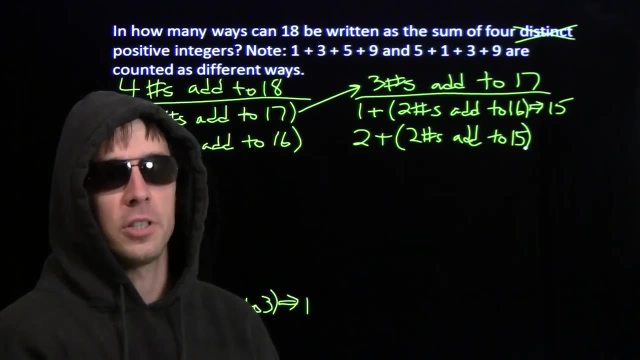 the second number. So there are 15 in this list. That's not too bad. And then you have 2 plus 2 numbers that add to 15.. Now, once again, this is a pretty easy list to count. You can take anything from 1 to 14 as the first number and you automatically have the 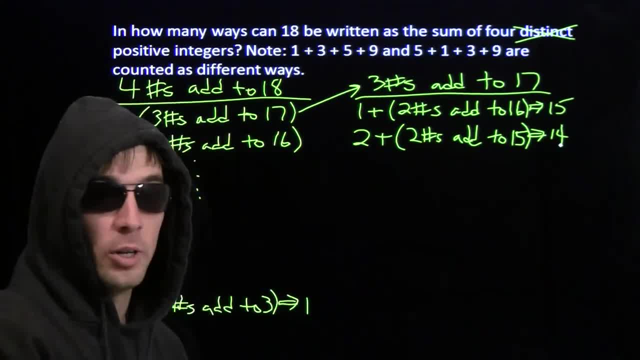 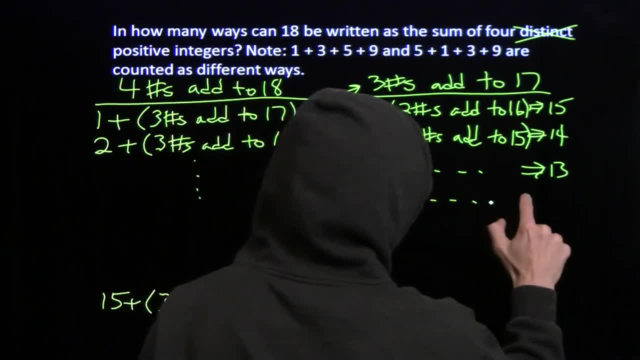 second number. So there are 14 ways to do this, And now you see where this is going. We start off with 3 plus da-da-da-da-da. There's going to be 13 of those: 4 plus da-da-da-da-da. 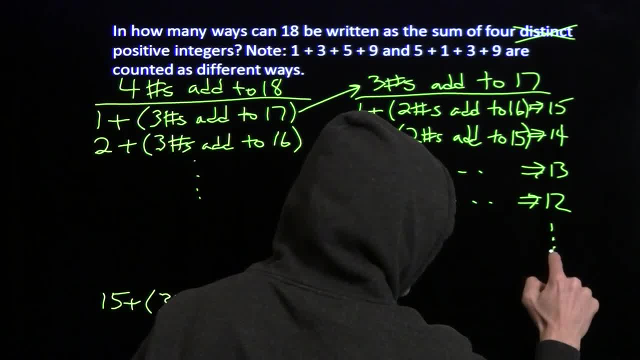 There's going to be 12 of those, And so on down the line. This will keep on going. Then you'll have 4.. Then you'll have 3.. Then you'll have 2.. Then you'll have 1.. 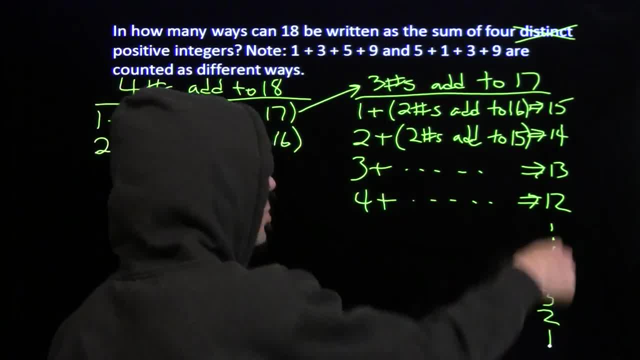 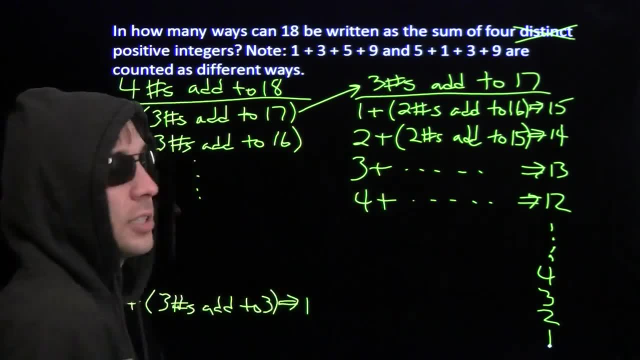 So the number of ways you can get 3 numbers to add up to 17 is 1 plus 2 plus 3 plus all the way up to 15. Whew Gets you that number right there, And then you've got to do it again for 16.. 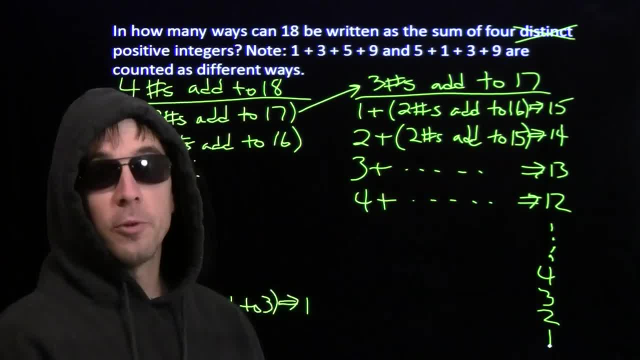 Right, there are 3 numbers that add to 16.. Of course, that will be add 1 all the way up to 14, and so on and so on. That's going to take forever, So we're going to work from the bottom instead. 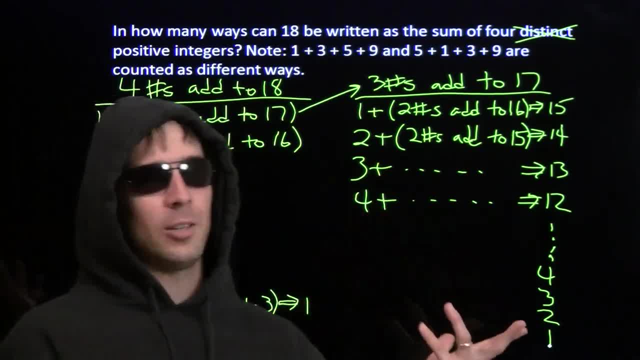 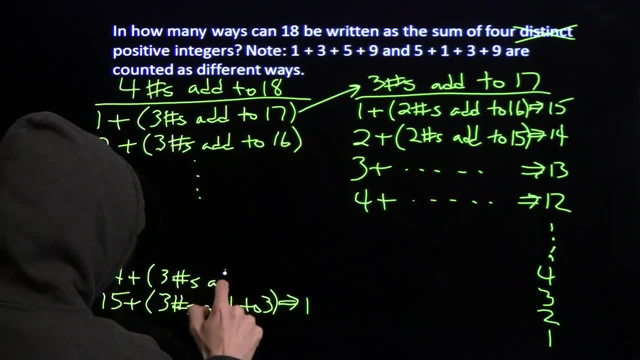 Start working from the bottom. Maybe we'll see a pattern. Maybe we'll already see the pattern. That's awesome. Let's start working from the bottom. 14 plus 3- numbers that add to 4. Doing something stupid can be a lot of work. 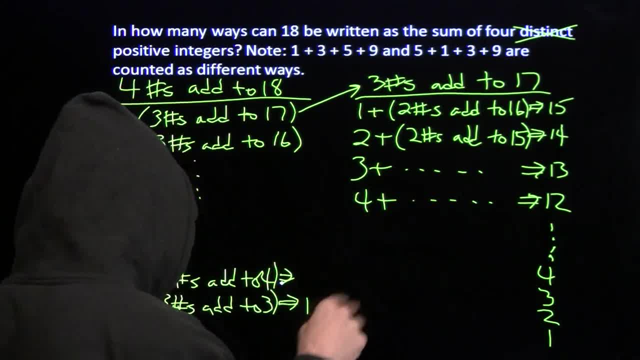 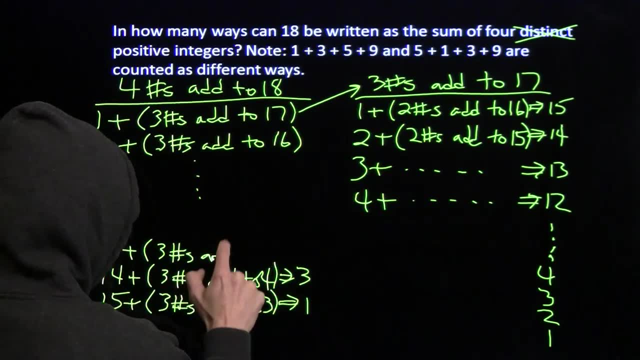 All right, 3 numbers that add to 4.. 2, 1, 1.. 1, 2, 1.. 1, 1, 2.. There's 3 groups right there. Let's try 13 plus 3 numbers that add to 5.. 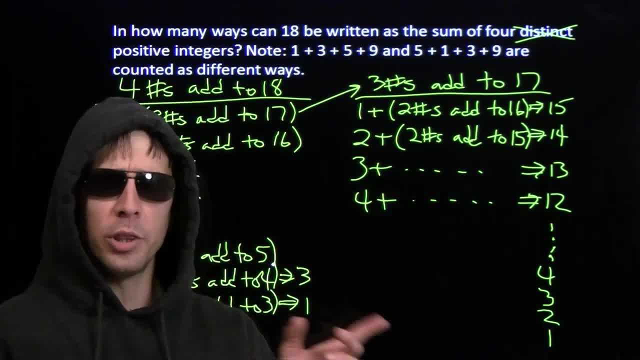 All right. 3 numbers that add to 5. 3, 1, 1. 1, 3, 1. 1, 1, 3. 2, 2, 1. 2, 1, 2.. 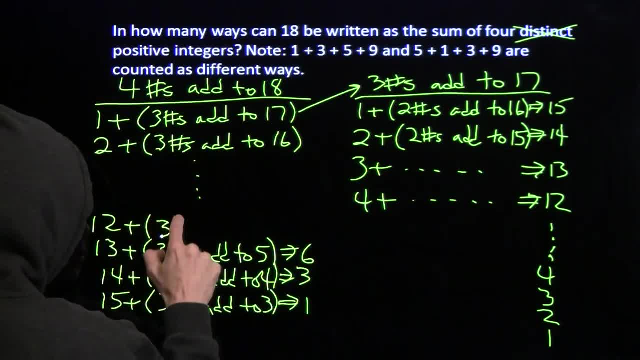 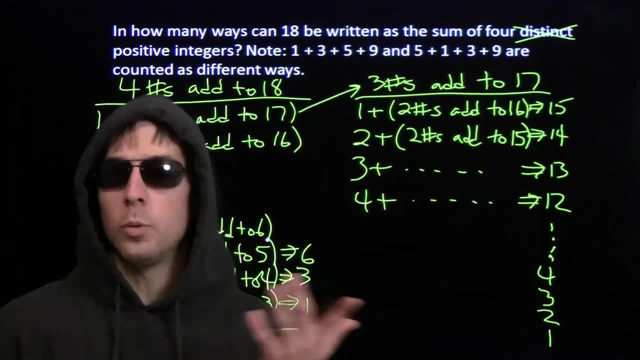 1, 2, 2.. There are 6 of those, Now 12 plus 3 numbers add to 6.. Let's see We got 4, 1, 1.. 1, 4, 1.. 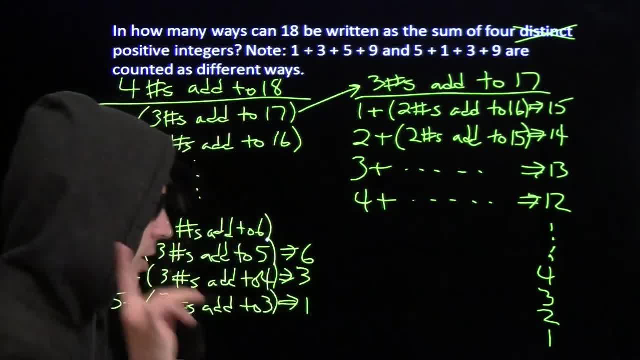 1, 1, 4.. Then you got 3, 2, and 1. There are 3 factorial 6 ways to order those 3 numbers, So that's 9 total, And then there's 2 plus 2 plus 2.. 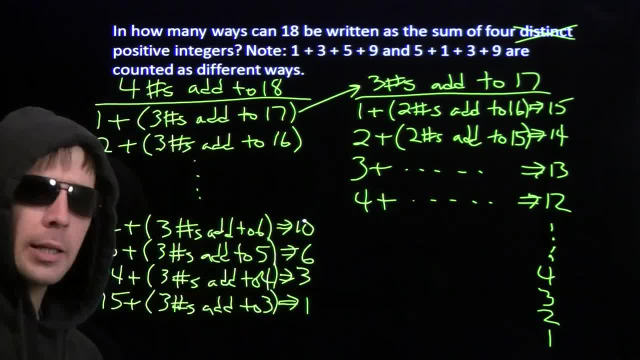 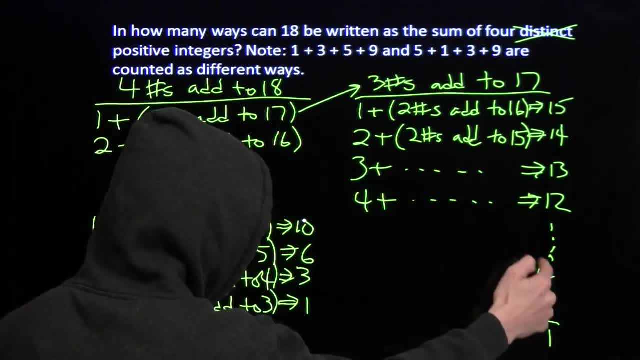 That gives us 10 ways to do this. Now maybe you recognize these numbers. All right, You can see this: 1 plus 2 is 3.. 1 plus 2 plus 3 is 6.. 1 plus 2 plus 3 plus 4 is 10.. 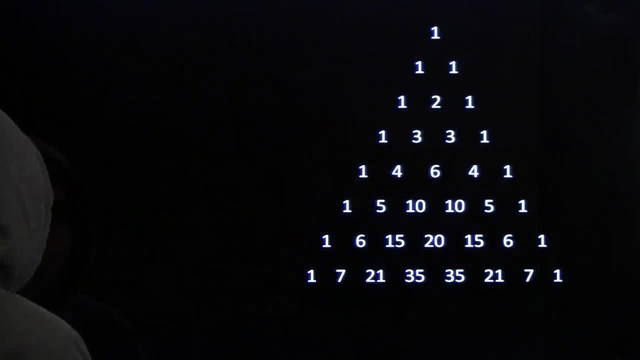 Or maybe you recognize these numbers from Pascal's triangle. All right, Now I would hope that the other guy would at least see this. He'd see that 1, 2, 3, 4,, 5, 6,, 7.. 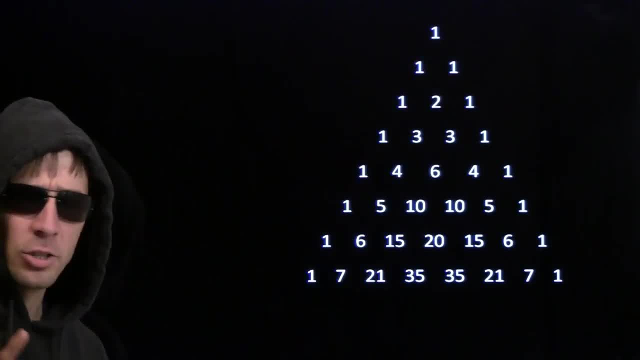 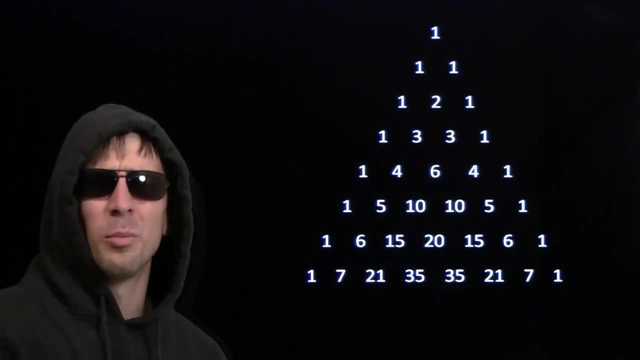 And he'd start thinking of this diagonal of Pascal's triangle. Once you start to see that 1,, 3,, 6,, 10, you start thinking of this diagonal right here And you start thinking maybe all these numbers come up on nice neat diagonals in Pascal's. 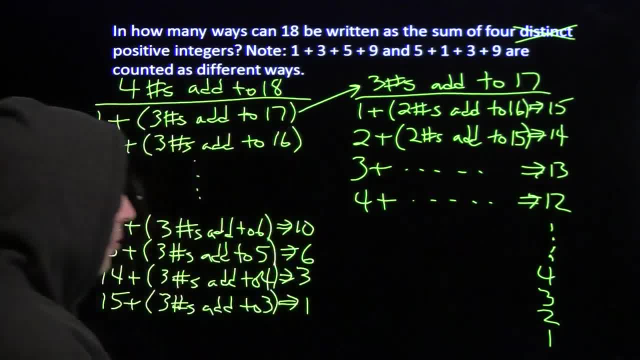 triangle. Take a look back here again. There's 1,, 2,, 3,, 4,, all the way up to 15.. That was one diagonal, And here's another: 1,, 3,, 6,, 10.. 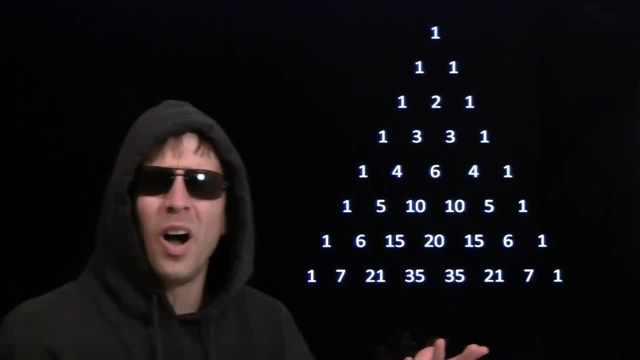 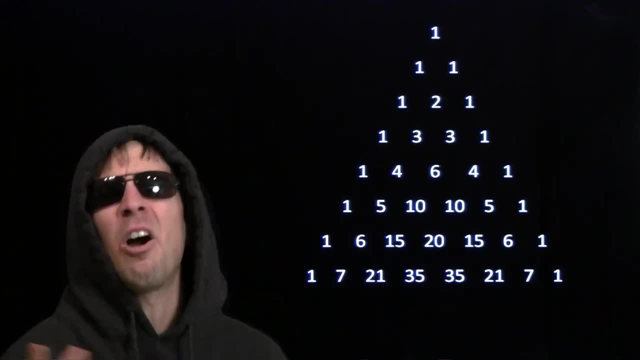 1,, 3,, 6, 10.. Right along that diagonal. What's going on? What's going on here? And this is where that other guy would really get stuck. You know why? Because his imaginary friend can't help him with this. because Harvey only knows geometry. 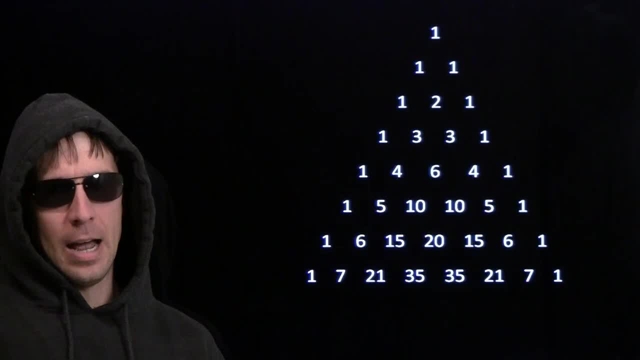 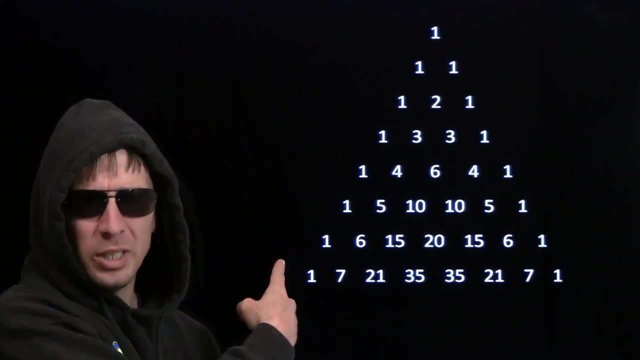 He needs me for this because, you see, I like to count And people who like to count when they look at Pascal's triangle, they don't see this. This is not what we see when we think Pascal's triangle. This is what we see. 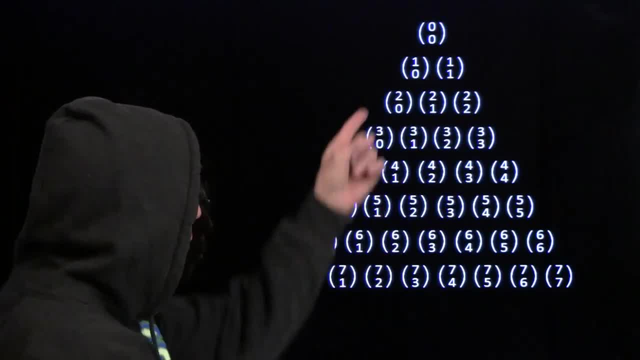 We see these binomial coefficients. We see 0, 2, 0 at the top, 1, 2, 0.. 1, 2, 1.. 1, 2, 0.. 1, 2, 0.. 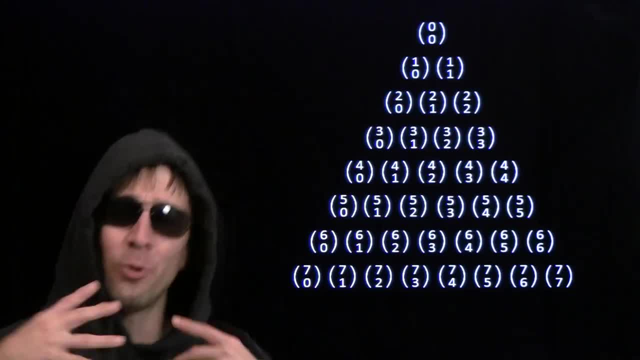 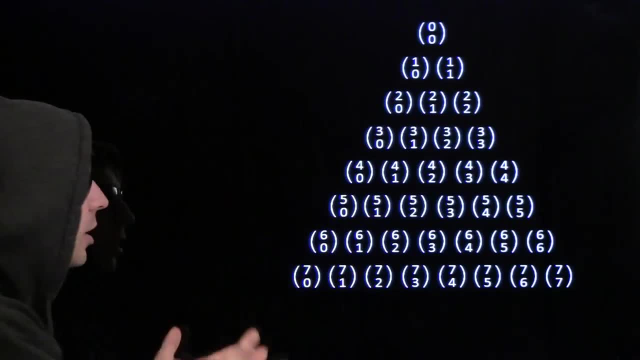 This is the way I see Pascal's triangle. Now, if you've never seen this stuff before, you gotta go talk to your teacher and say, hey, show me the good stuff, because this is some good stuff. This is Pascal's triangle right here. 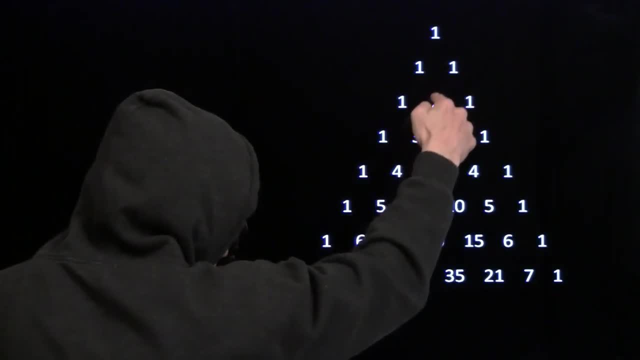 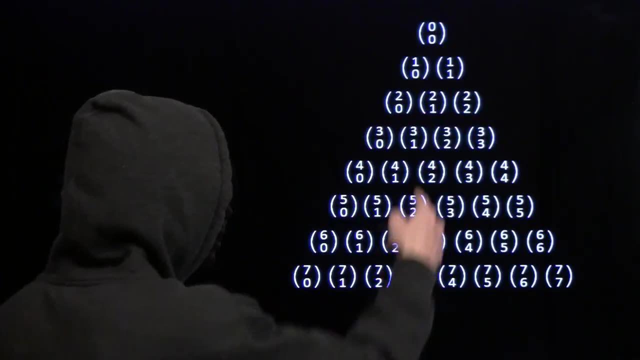 And this diagonal right there. that's these numbers right here: 1, 2,, 3,, 4,, 5,, 6, 7, that's these right here. That's the numbers, different numbers, of way you get two numbers to add up to something. 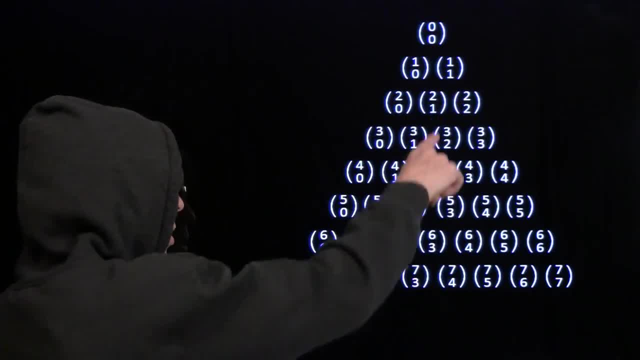 right there, Two numbers that add up to 2.. There are two ways to get two numbers to add up to 3.. numbers to add up to 4,. 2 numbers to add up to 5,. 2 numbers to add up to 6, then we went. 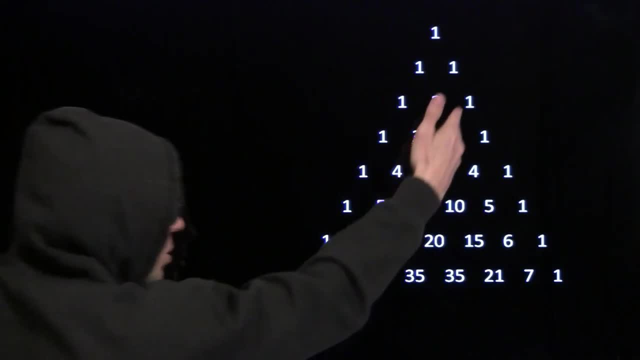 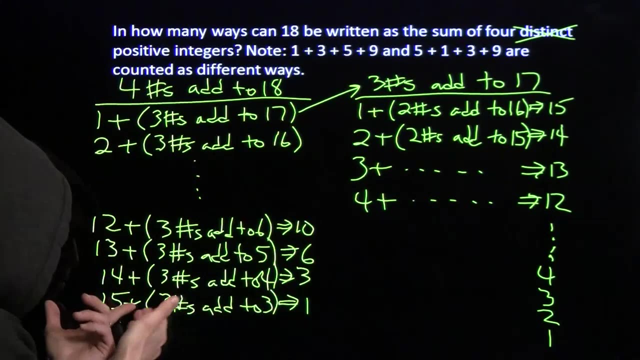 along this diagonal right here, That is, these numbers: 1, 3, 6, 10,. 1, 3, 6, 10,. number of different ways. you have 3 numbers to add up to something, 3 numbers to add up to 3, 3 numbers to add up to 4,. 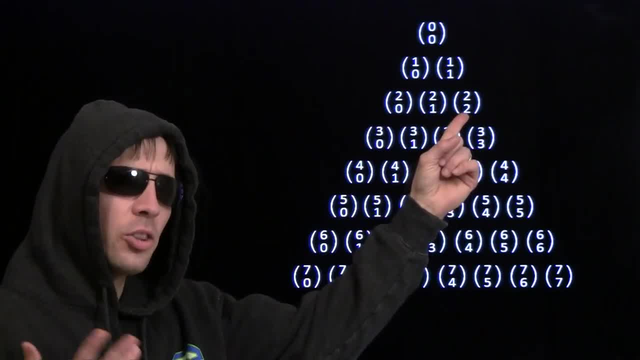 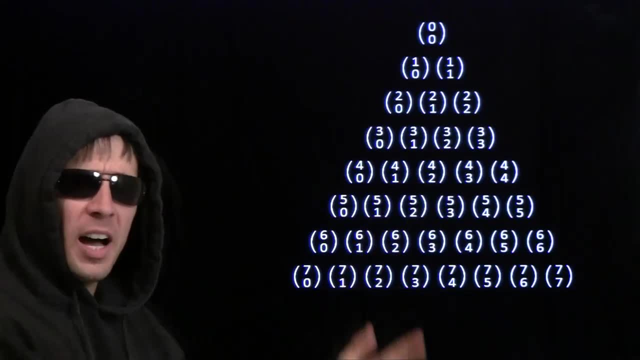 right along this diagonal. There's 2: choose 2 ways to get 3 numbers to add up to 3.. There are 3: choose 2 ways to get 3 numbers to add up to 4,. 3 numbers to add up to 5,. 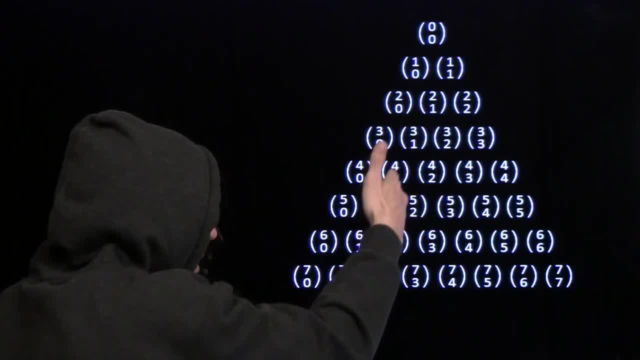 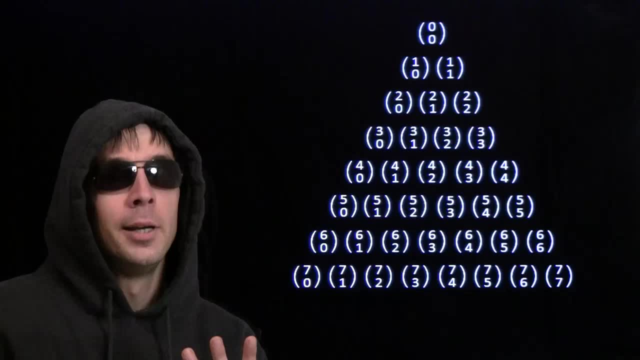 and so on along this diagonal. So here's the diagonal for all the ways you have two numbers to add up to something. Here's a diagonal for all the ways you have three numbers to add up to something. So we know where to go. looking for four numbers to add up to something, That's. 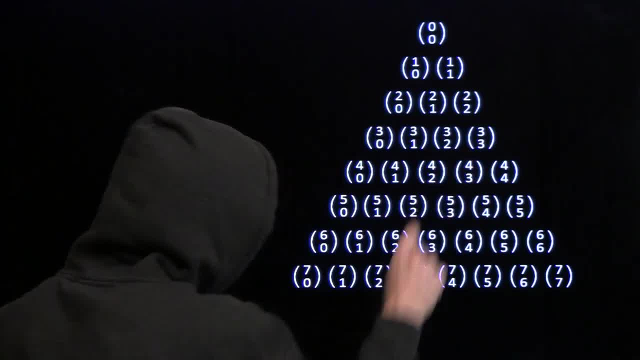 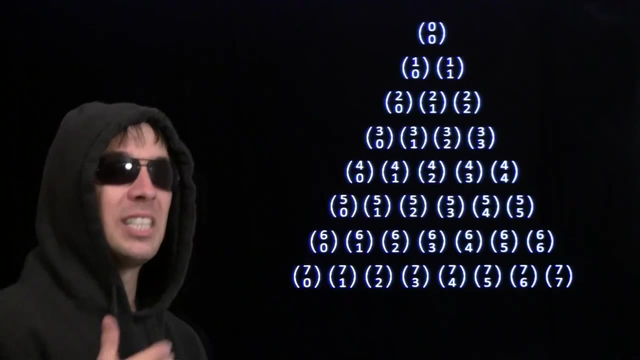 right along this diagonal here. Four numbers to add up to four. Four numbers to add up to five. Four numbers to add up to six. Well, there are five choose-three ways to get four numbers to add up to 6.. There's 6- choose 3 ways to get 4 numbers to add up to 7.. 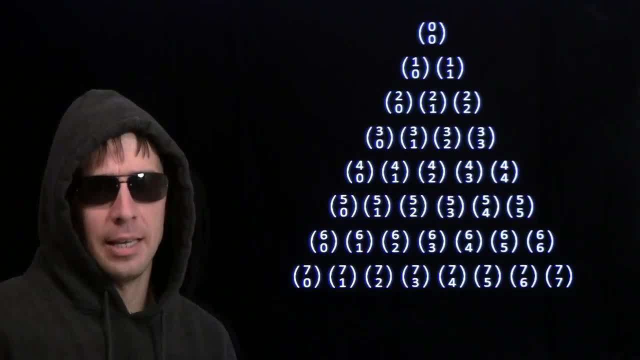 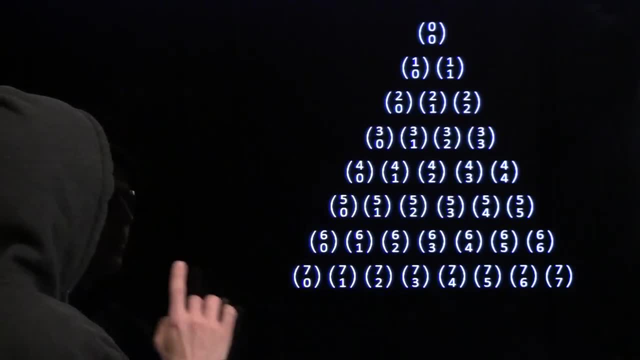 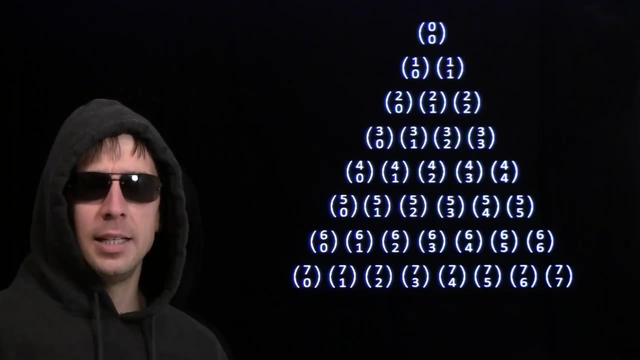 Well, we want 4 numbers to add up to 18.. There's probably 17. choose 3 of them. This looks like a pretty good guess, but we don't like guessing, we like knowing. Why are there 17? choose 3 groups of 4 numbers to add up to 18?. 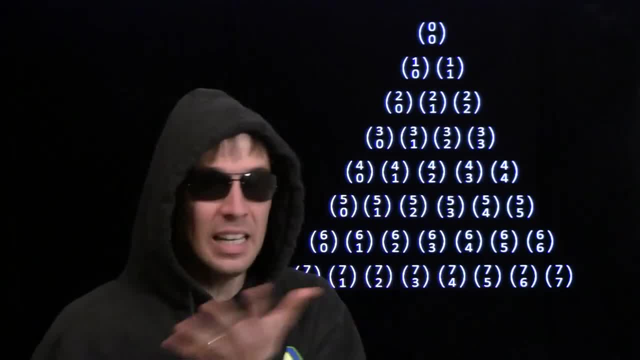 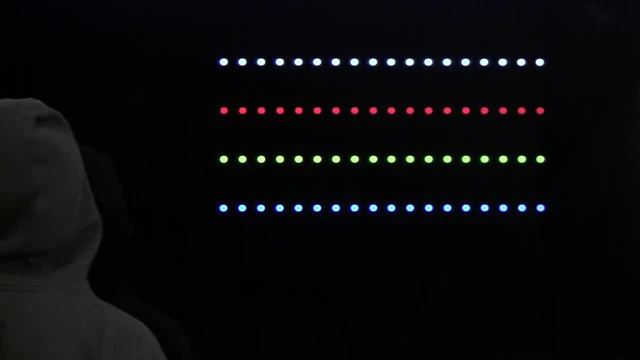 We've got to find some way to think about this problem, where we'll have 17 things of which we have to choose 3.. And this is what we're going to do. We're going to start off with these pretty dots. Now, each one of these rows has 18 dots, and if you don't trust me, you can pause the video. 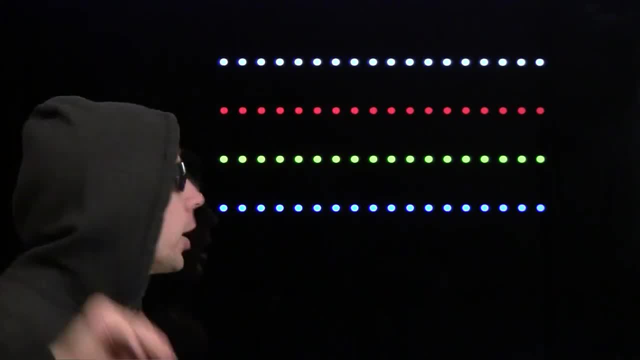 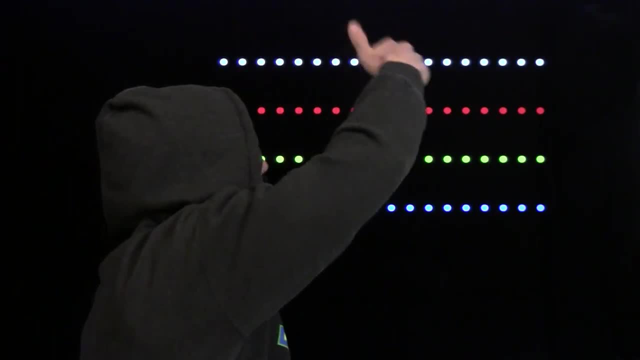 and count them, Or you can just stop listening to me and count them while I'm talking. Look at this first row. There's 18 dots. What is there 17 of? There's 17 spaces between the dots. Well, let's choose 3, because we think 17 choose 3 is the answer. 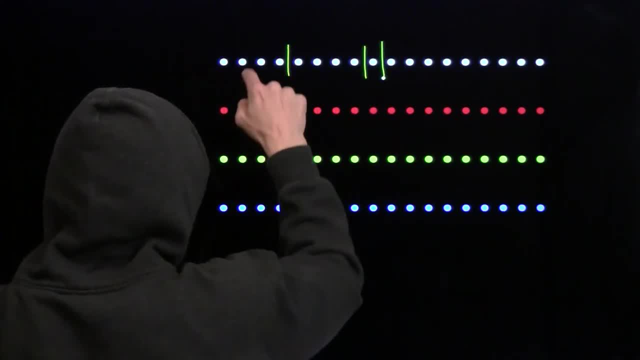 I'm going to choose 3.. I'm going to choose these: 3. And look at that Right over here, 4 dots Right there. 4 dots Right there. 1 dot Over here there's 9.. 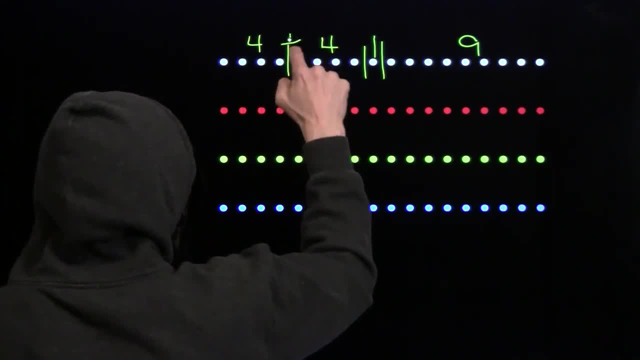 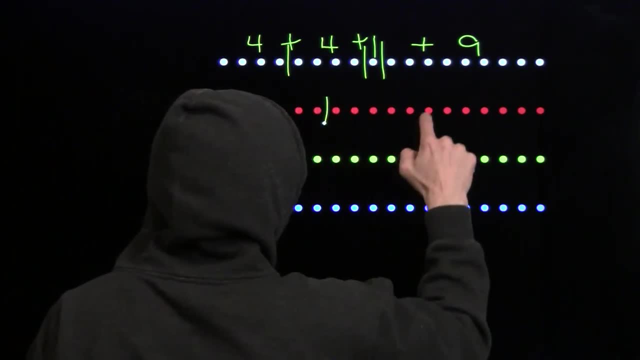 4 plus 4 plus 1 plus 9.. Add these 4 numbers and of course you get 18.. There are 18 dots up there. Let's try it again. We'll put it there, there and there. 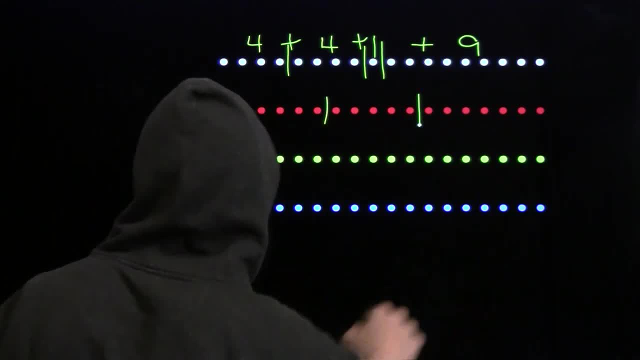 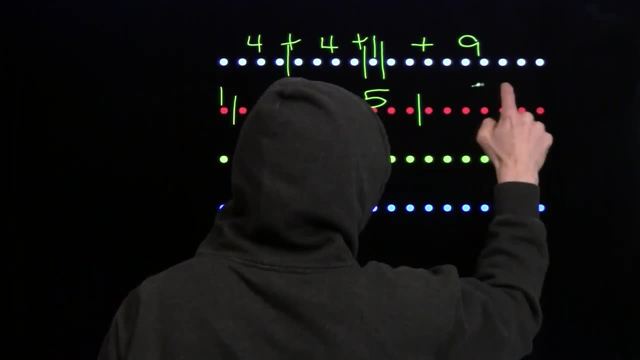 That's where I choose. I chose those 3 blanks to put bars in out of these 17.. One dot over there. Five dots there. Five dots there. One, two, three, four, five, six, seven dots there. 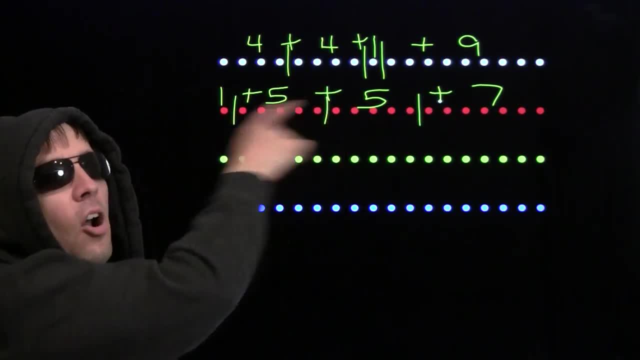 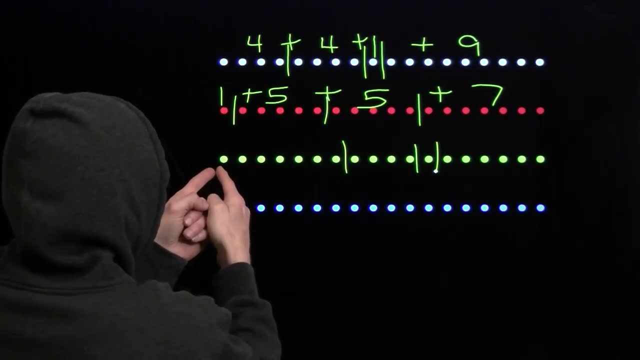 One plus 5 plus 5 plus 7.. That's 18, because there are 18 dots. All right, I'm going to do this two more times. make sure I'm not doing anything too silly. Let's see, We got 3 and 4..